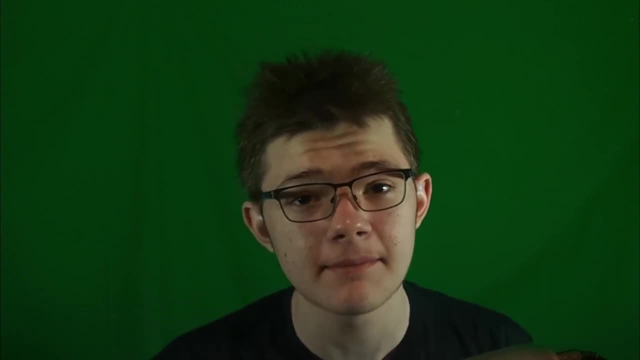 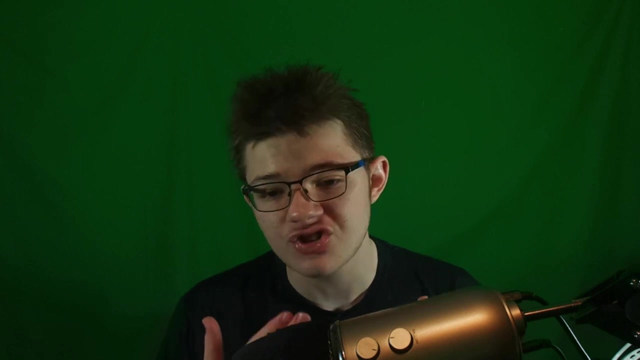 should I honestly care about coastal erosion? It has nothing to do with me and it might not even affect me at all, so why should I care about it? Well, coastal erosion is actually something that is going to change a lot of things throughout our life and, believe me, it's already happened. 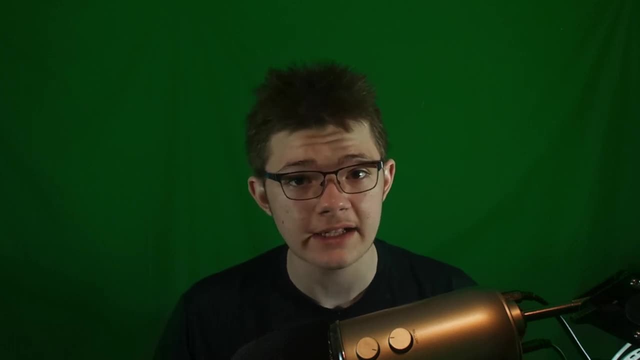 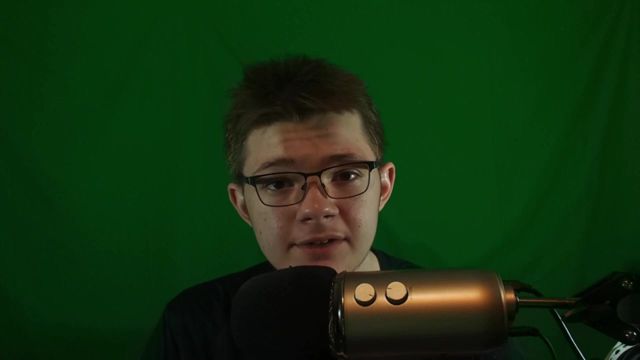 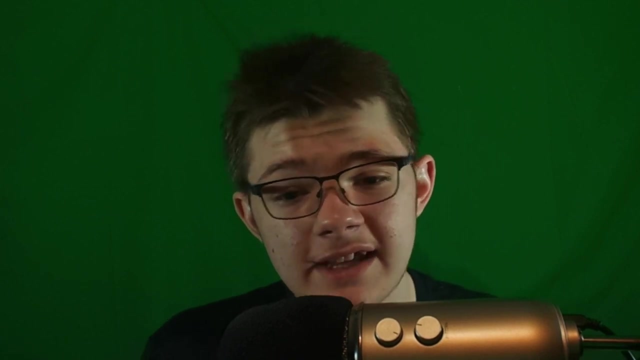 It's already happening around the world. Prime example is Venice, Italy, It is said, based on data. every single year the city sinks two milliliters. each year the water rises. Now you're probably wondering: why should we honestly be scared about that? Well, it's common sense. By 2100, it is said. 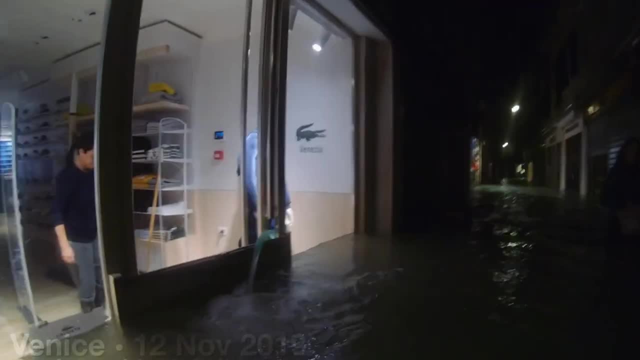 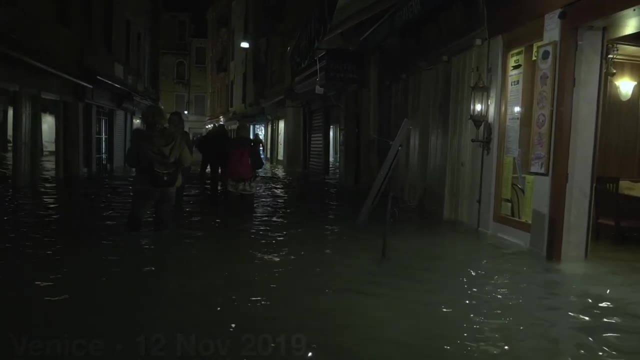 that Venice will be submerged underwater. Now the issue with that is, when you think about it, it's not that far away. It really isn't. It's not that far away at all and we're talking a whole city being submerged underwater because of something. 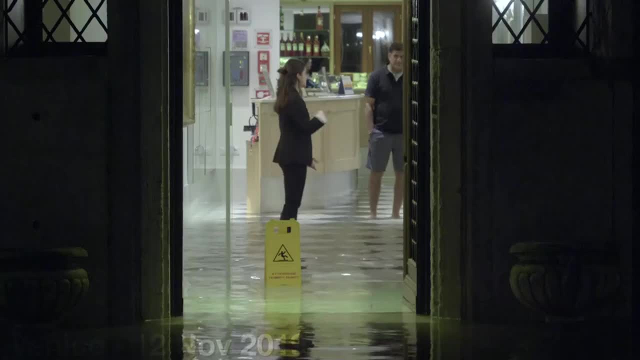 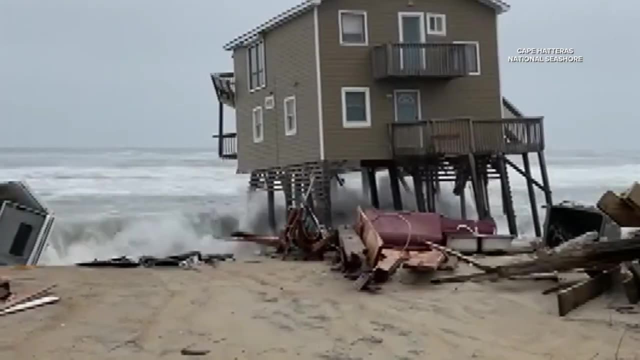 that we could possibly fix with some sort of way that I'm going to talk about later on. But another prime example of this is also what's going on in the Outer Banks Here, as you can see in this video, a whole house just being completely destroyed by coastal erosion because, well, the sand sinks and 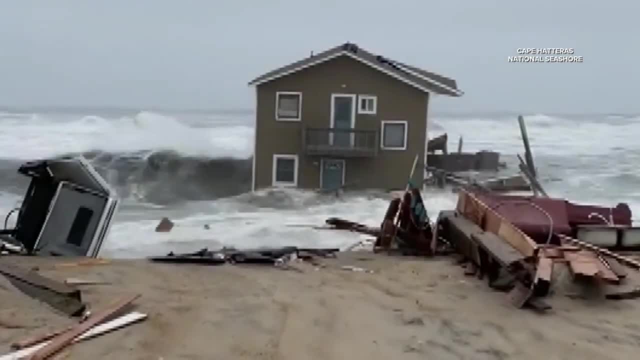 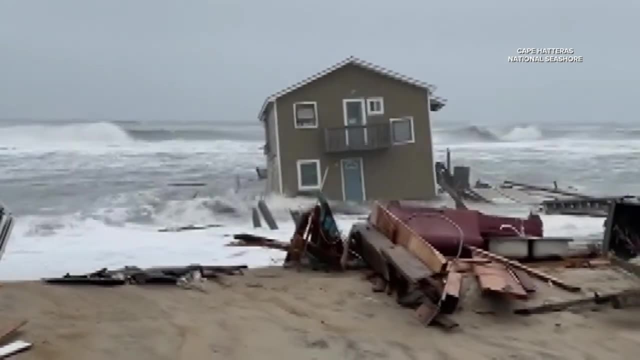 water rises, and so what happens? there's no land for that house anymore, and so what happens? well, I think you know, the rest house gets submerged underwater and it's completely destroyed. Now, if you're on the coast, you probably should be worried about this, because this is a really 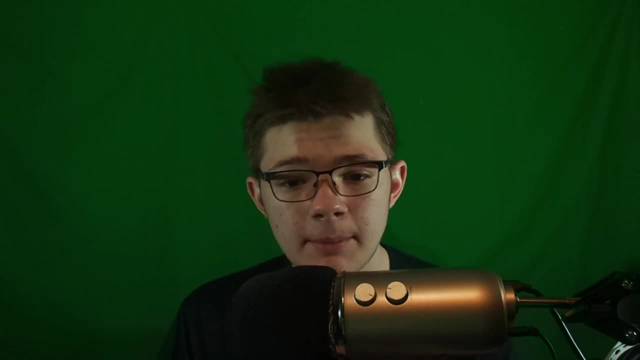 serious thing. It can even happen on lakes. It also can happen on rivers as well, especially with floods and all that stuff as well. So the question is: what is the solution to coastal erosion? Well, let's talk about it. So one of the first solutions to coastal erosion are obviously sea. 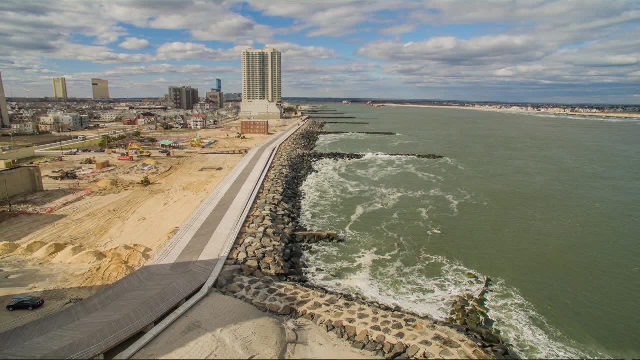 walls. Now, sea walls are really popular because of the fact that they are actually really strong and they have a very long gativity. These solid structures are typically made of concrete, which means they can withstand a lot of wave energy. Sea walls are often topped with a walkway or 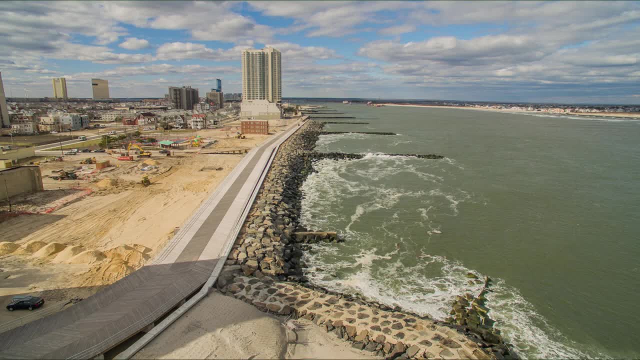 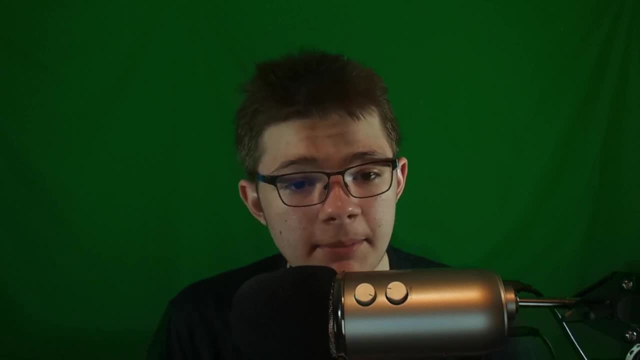 boardwalk, which means they can also do double as a sight seeing locale. Now you're probably wondering what is the other solutions? Well, I'm going to talk about them as well, But sea walls are something that we really should invest in, especially here on the outer banks. 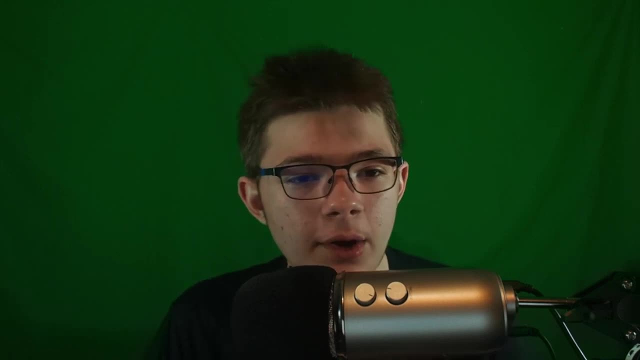 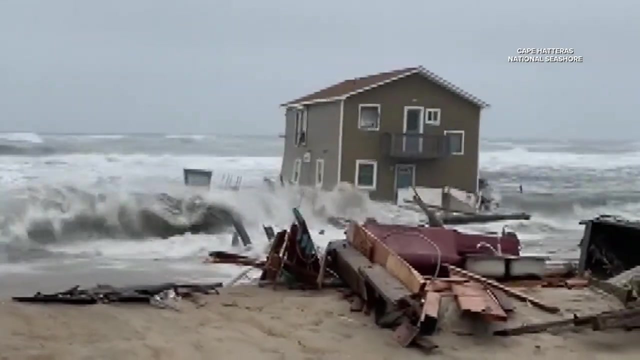 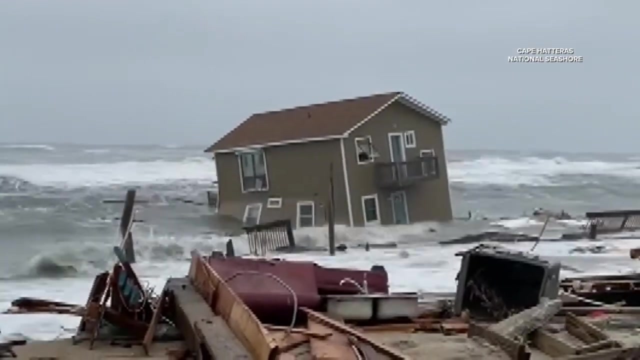 in this country because we are seeing houses, we're seeing buildings completely washed away because the water is rising to the point where there's no land for that house or the building to even be, and so eventually, when the time comes, that house is washed away because the water. 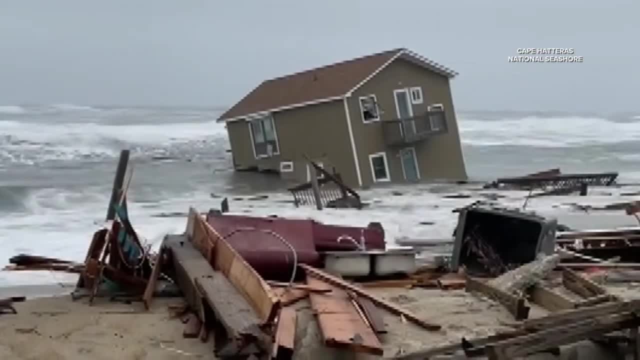 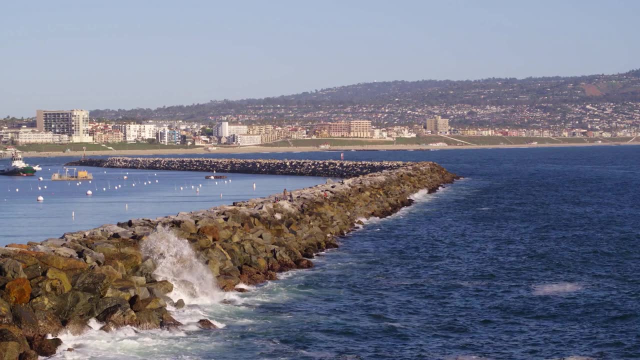 just ends, does exactly what it did in the video I just showed you. So that is one of the solutions. The other solution is, of course, breakwaters. Breakwaters are stone structures that protect the coast and harbors from wave erosion. These revetment systems stand in the water and breakwaters. 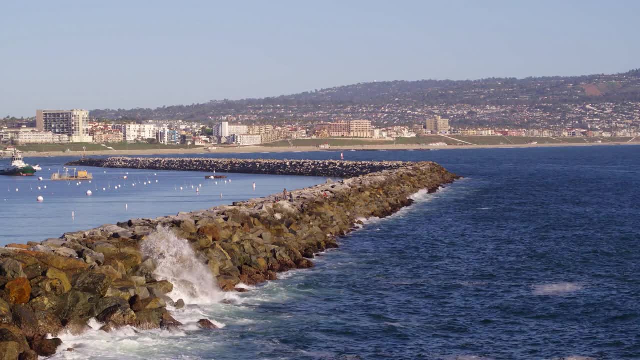 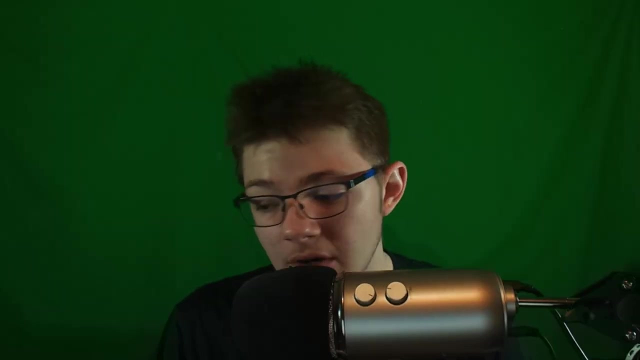 can be parallel or perpendicular to the shoreline, So that would actually help a lot and, honestly, there's a lot of advantages with them. The fact that they are parallel to the shore are often found in the water outside of small harbors and beaches. They protect these vulnerable environments from erosive wave energy, So that could possibly be. 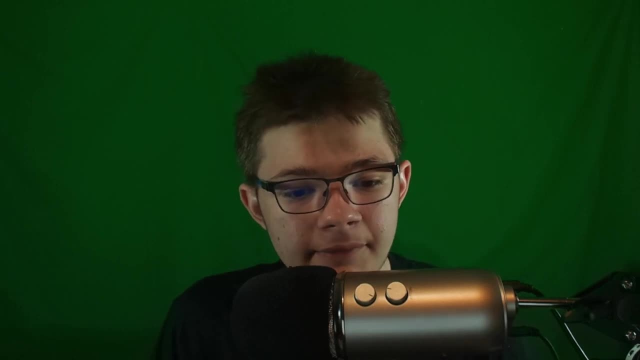 another solution Now, another one we possibly could think of is, of course, sandbags, geotubes and dune stabilization, and possibly maybe even just fixing up the beach is another thing you want to do. Maybe add a little bit more sand onto it and just completely reconfigure the whole beach. 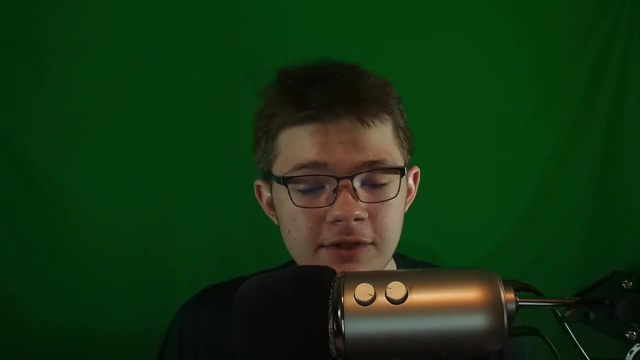 and add some sand to it, You know, add some defenses from the water so that it can't go that far and can get to the houses or buildings that are on the beach. So yeah, that's all I wanted to talk about today. I appreciate y'all for tuning in. If you guys did enjoy, let me know by dropping. 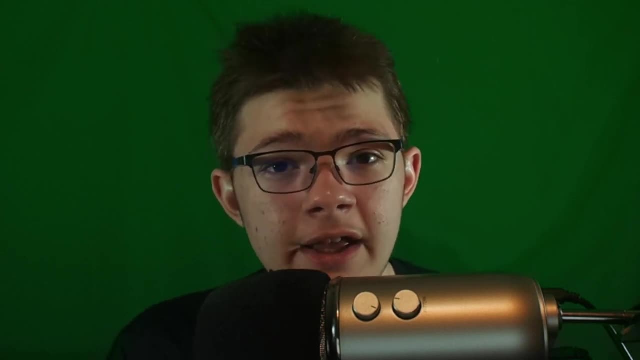 a like and thank you once again, Ms Costell, for being a great teacher. Appreciate everything you've done for us this year. Thanks for the, of course, the, the starbursts and skittles for our last class of the year. Appreciate it. Hope you have a great summer and have a great one. Goodbye.